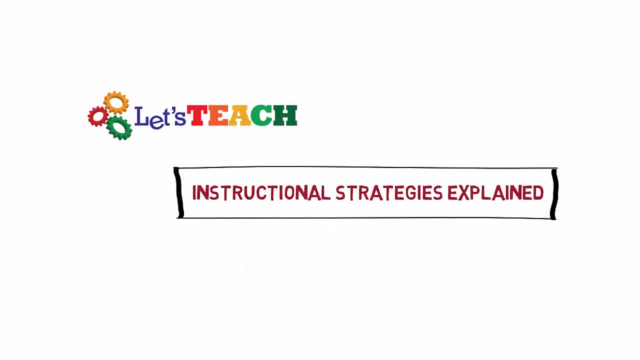 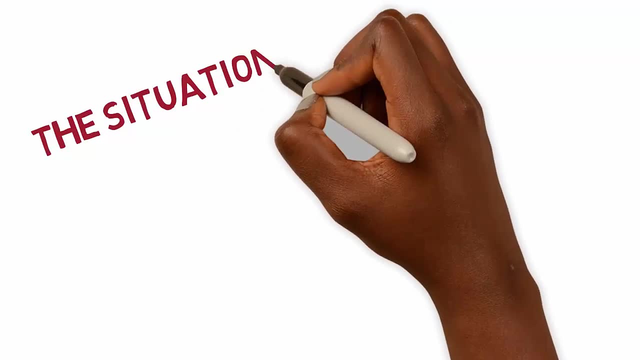 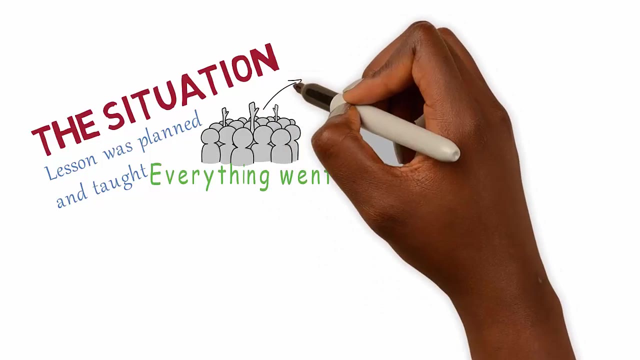 Here's a situation: You planned a great lesson and presented it to your students. As far as you could tell, everything went really well. The students were listening intently as you spoke and there were virtually no behavior issues during the lesson. You're especially 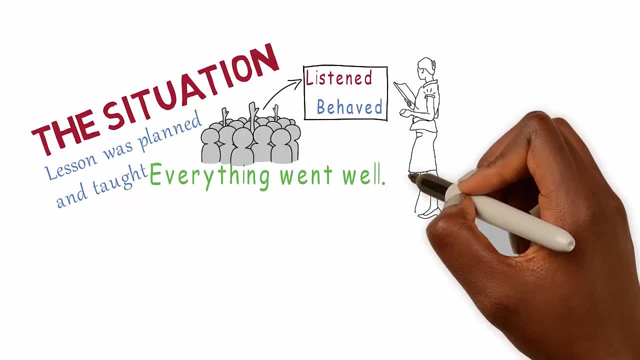 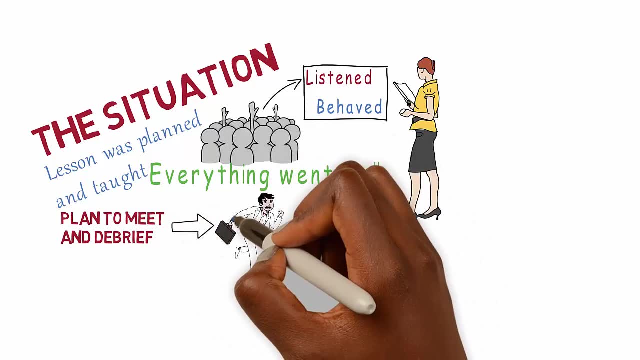 happy with how things went because your principal was observing the class. You and your principal decide to meet after school to talk about how the lesson went, so you hustle to the office to get her feedback. The principal lets you know that the lesson went really. 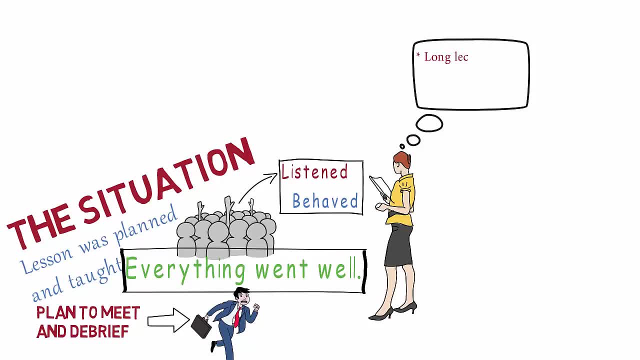 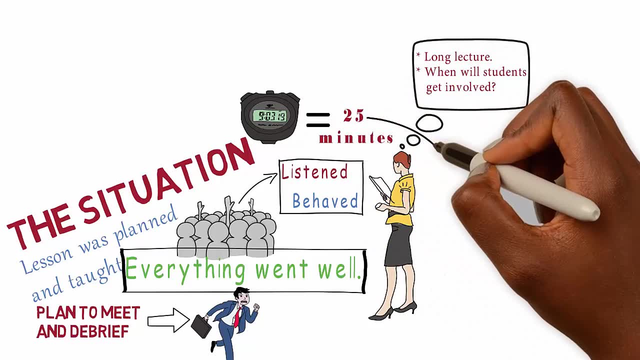 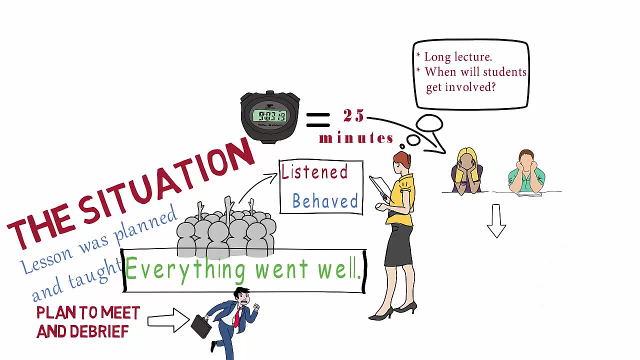 well, but has one big issue. She says you lectured for too long. She actually timed you and said that you talked for about 25 minutes of the 60-minute class. She also points out that this means for 25 minutes. students weren't really given an opportunity to ask questions. 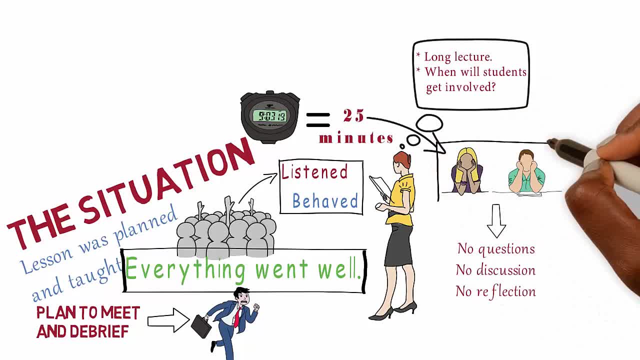 discuss anything or reflect. The principal goes on to say that during the next observation she would like to see students more involved in the learning process. She then offers this thought: The person doing the most talking about a concept is probably doing the most learning about it. 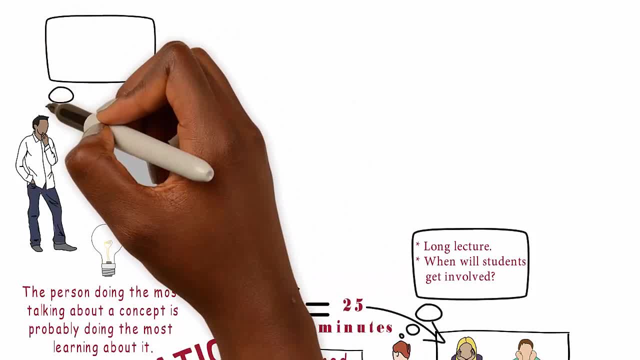 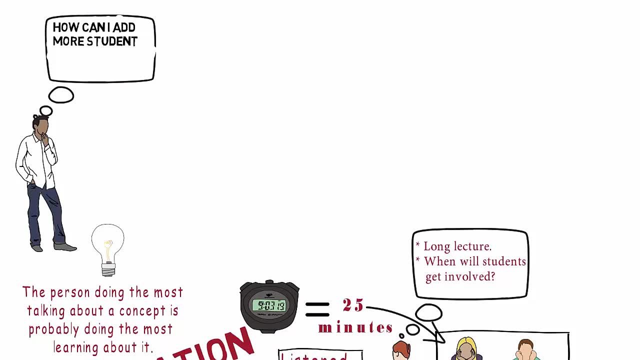 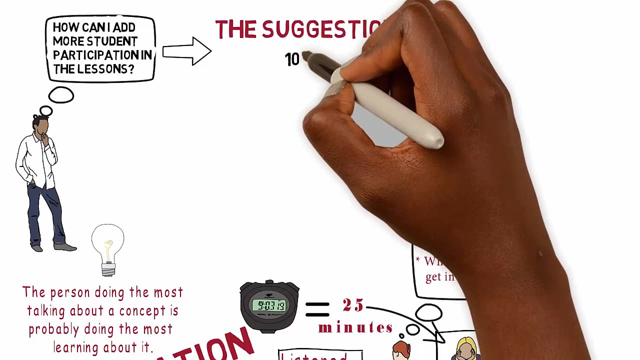 As you reflect on the meeting, you understand that the content of the lesson was good, but student participation was lacking for too long into the class. You need a strategy to make sure students are involved during the lesson itself. Allow me to offer a suggestion. Consider 10 plus 2.. No, not the math problem, the teaching. 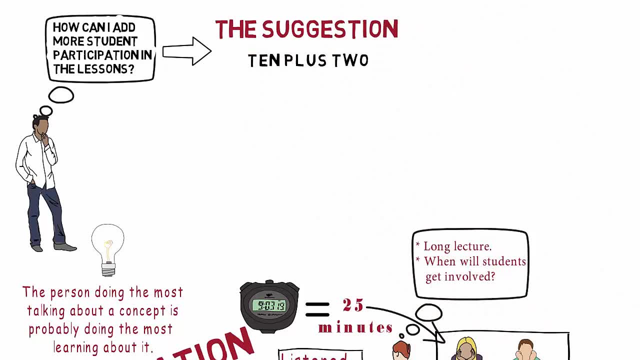 strategy 10 plus 2 is actually a direct instruction teaching method that works really well for teachers who are looking for ways to make sure students are active participants in the lesson. Here's how it works: The teacher provides direct instruction for about 10 minutes and 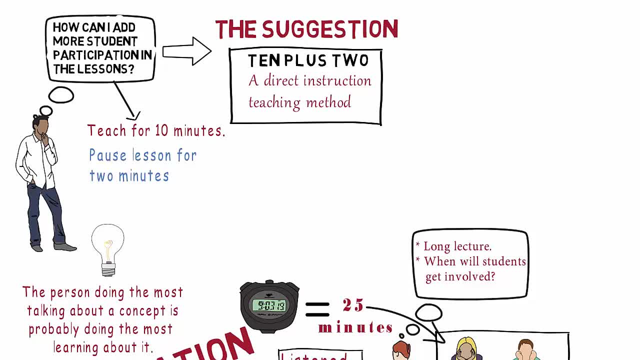 then pauses the lesson for 2 minutes. During the 2 minutes, students can do a variety of things. For example, you could have them do a quick journal entry about what they've learned up to that point in the lesson. You could also ask students to partner up and